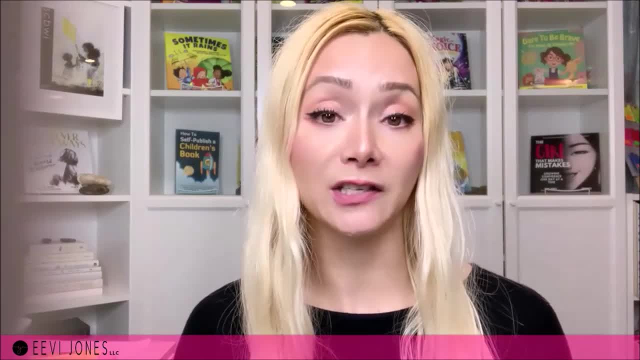 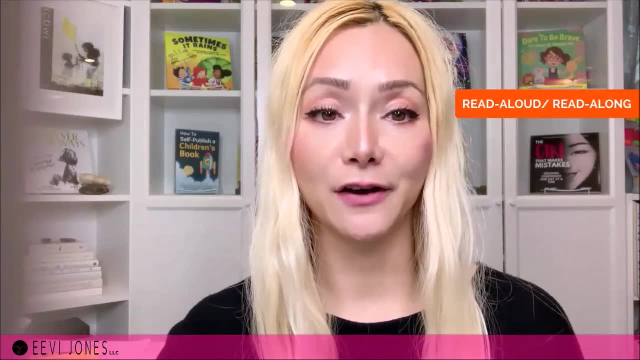 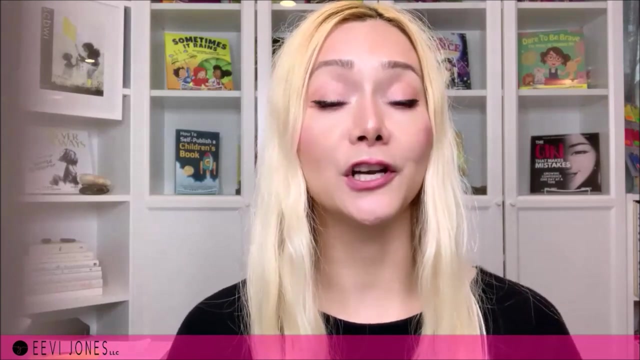 this. so in this video, I'm going to share one of my favorite ways, using two tools that are easy to use and absolutely free. So what are read-aloud or read-along videos? Here's what they are not. Read-along videos of our books are not book trailers. I made a whole, separate video on just. 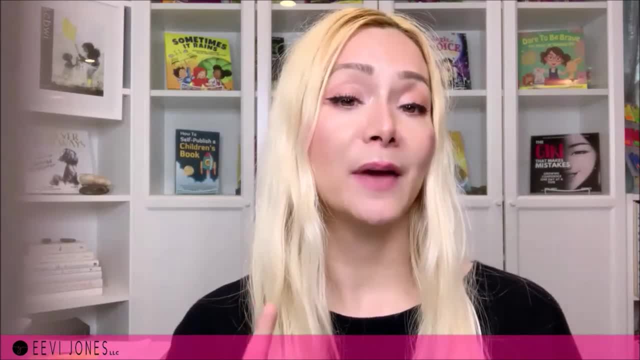 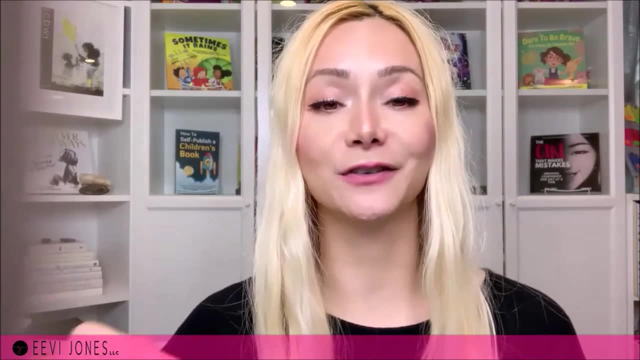 book trailers what they are, best practices and the main resources I would recommend if we want to create our own book trailer. I went ahead and added the link to that video in the description below. Book trailers are very much like movie trailers. They are little snippets or teasers. 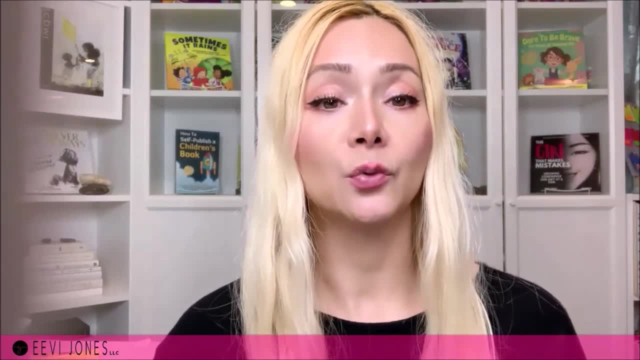 that we can share to get people interested in our book. Read-aloud videos, on the other hand, are videos where a book is read in its entirety. Oprah Winfrey said that reading a book out of a book. in work, I would like to try to use the materials I use and maybe use a hasheshghant, so I think maybe this would be a better way to 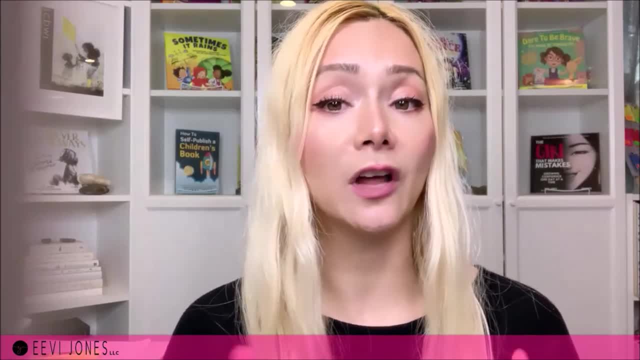 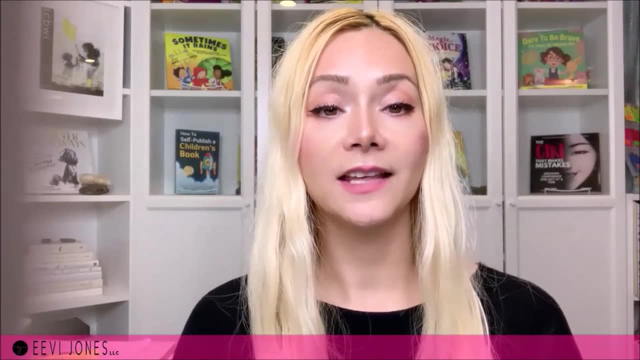 Read Aloud has had such a big moment during the pandemic, where lots and lots of people recorded themselves reading children's books to be watched and shared on platforms like YouTube. These types of videos work especially well with picture books, less so with middle grade chapter books. 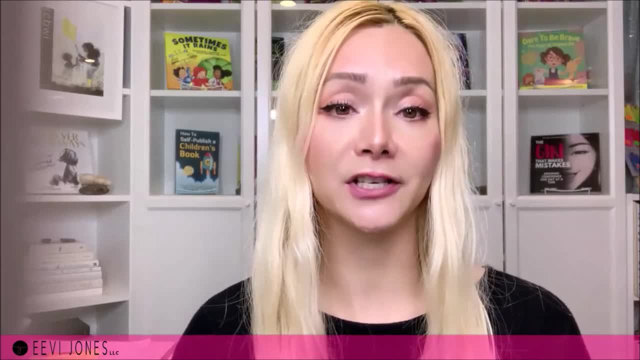 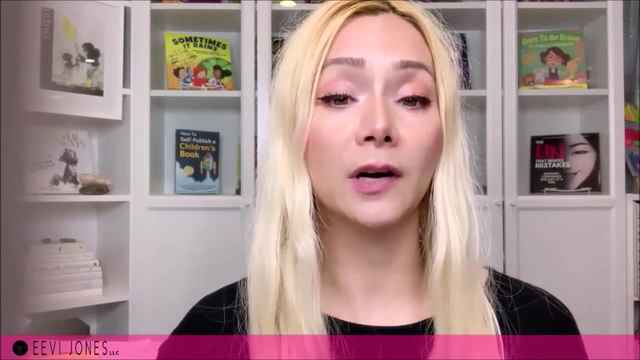 And that's because, one, picture books have lots and lots of illustrations to focus on during the Read Aloud And, two, because picture books are relatively short, we can read the book out loud in less than five minutes, which is perfect for little readers. 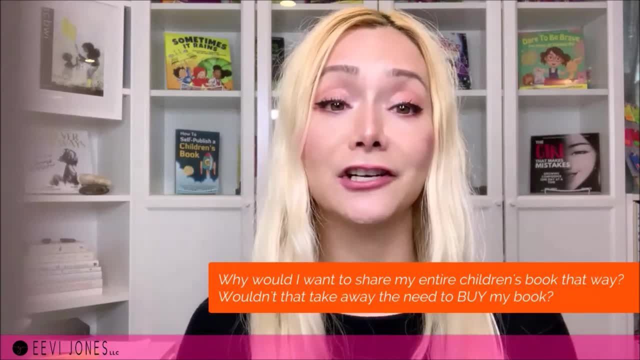 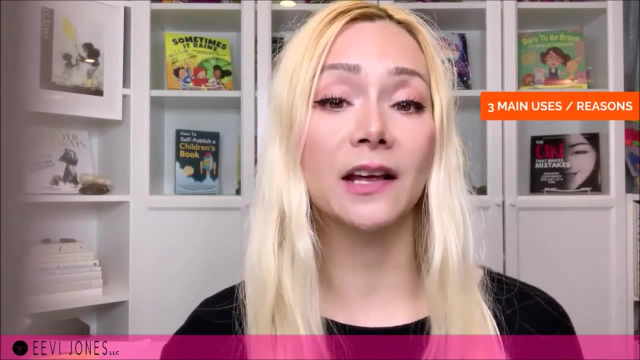 Now you may be asking: but Evie, why would I want to share my entire children's book that way? Wouldn't that take away the need to buy my book? So let's look at the three main reasons why creating a Read Aloud video can be really. 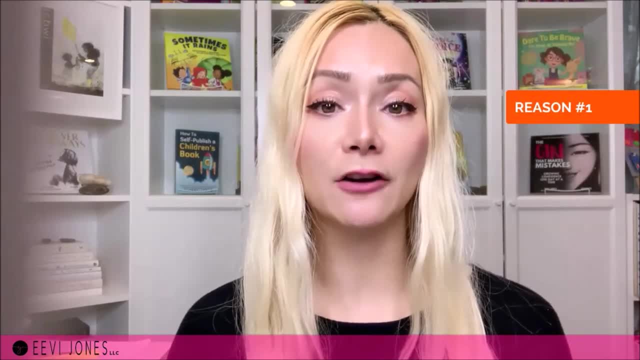 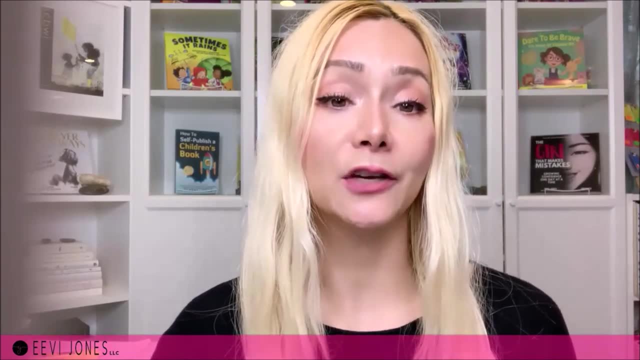 beneficial Reason number one is that we can use the Read Aloud of our book as a free marketing tool, Very similar to a book trailer. we can share our Read Aloud video on big platforms like YouTube. YouTube, just like Google, is a humongous search engine. 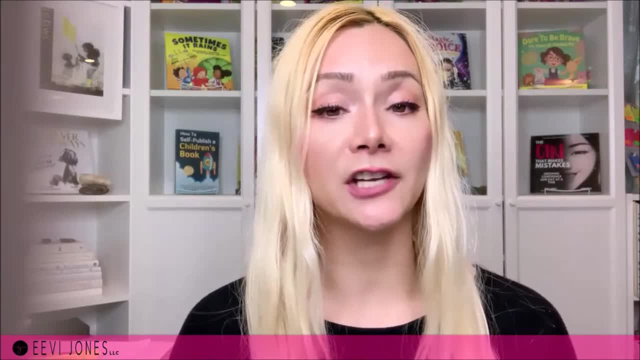 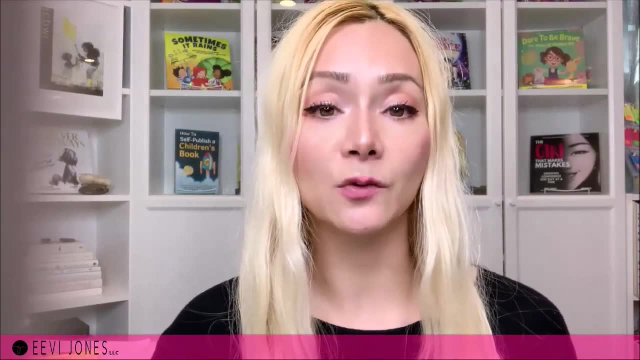 So with a Read Aloud video, we essentially get to attract potential eyeballs absolutely free. Now, if you're worried that this might stifle your sales, consider this Whenever someone finds and watches our Read Aloud video on, let's say, YouTube chances. 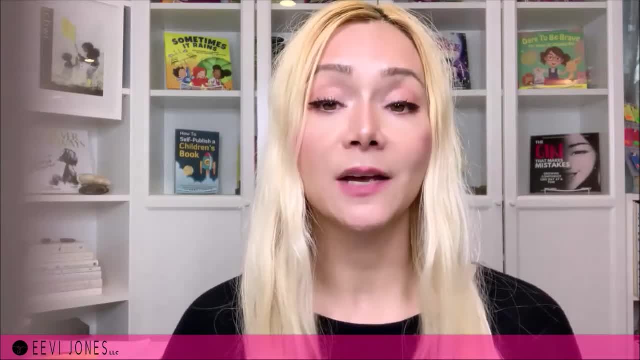 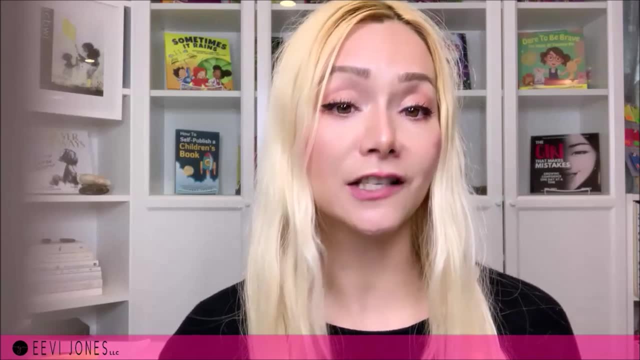 are very high that this person has never heard of us before, right, Meaning before that video. they probably didn't even know about us and our book at all, So it is usually because of our video that they learn about us in the first place. 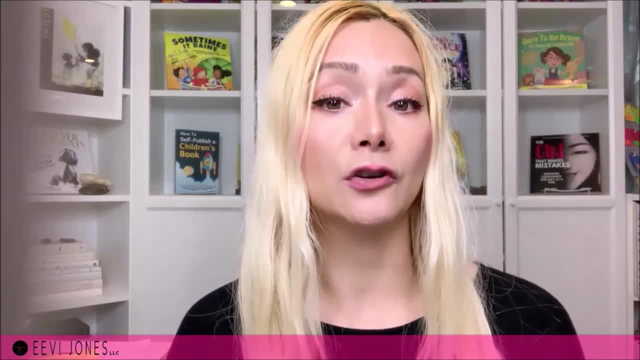 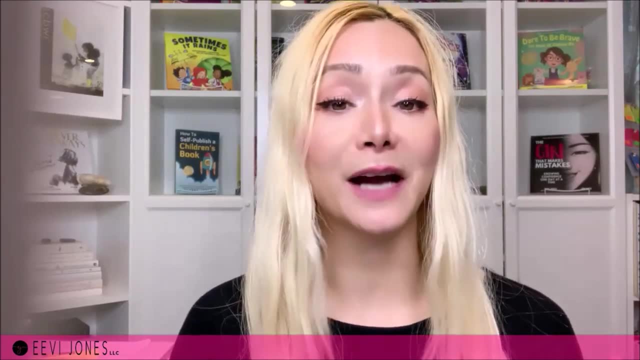 And after having found and watched our video, they probably didn't even know about us and our book at all. So they can now decide whether or not they liked it enough to go and buy it. And I am such a prime example that this test driving method really works, because I have 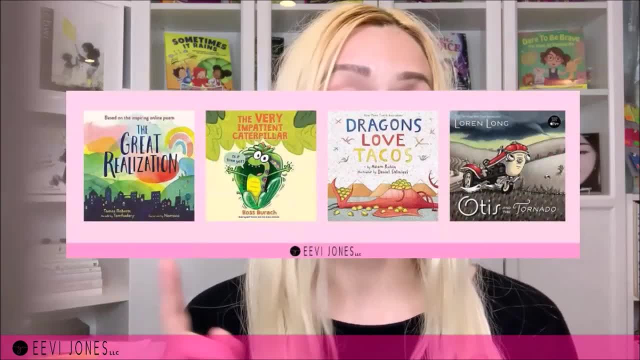 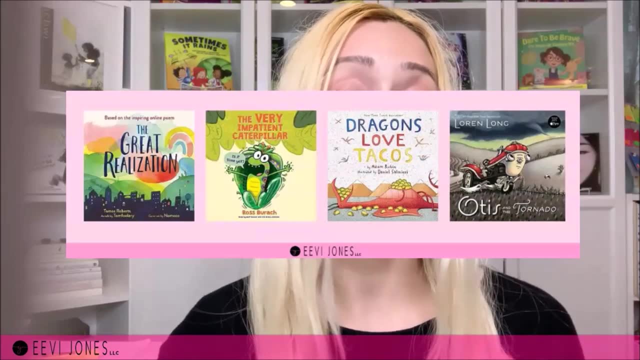 found and bought so many children's books that way, with The Great Realization, The Very Hungry Caterpillar, Dragon's Love, Tacos and Otis and the Tornado just being a few of them. Their Read Aloud videos didn't prevent me from buying these books. instead, they helped. 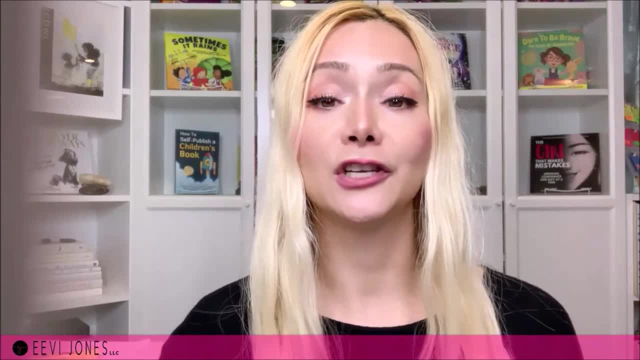 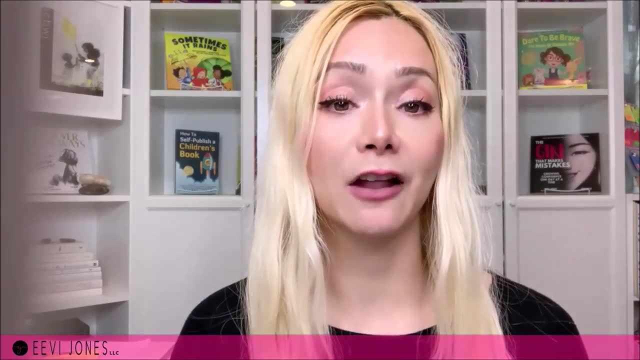 me discover them And like them so much that I went out to buy them, And so sharing our book that way is very similar to libraries in a way, just on a much, much greater scale of reaching people with a much higher potential of being found. 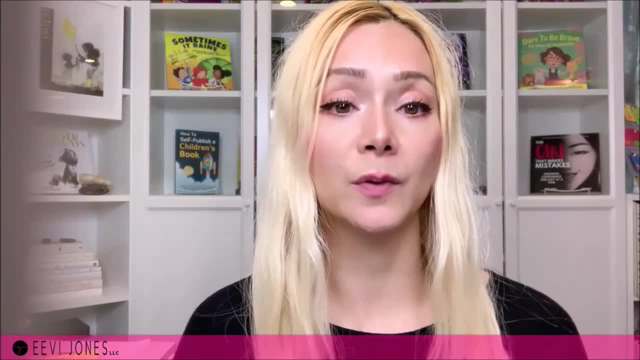 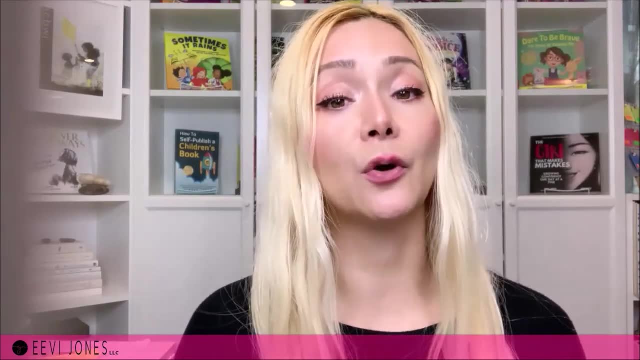 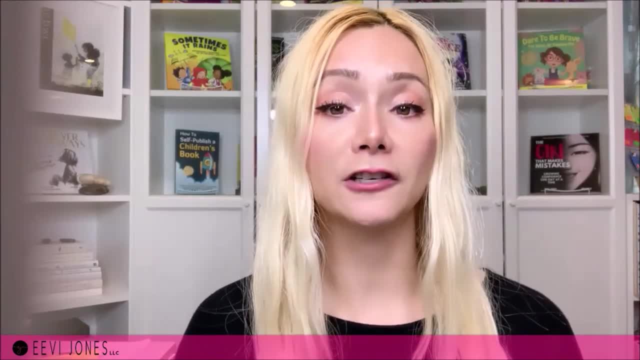 We can use the Read Aloud video of our book as part of our book. We can use the Read Aloud video of our book. We can use the Read Aloud video of our book as part of our book launch strategy. Something I love to do for the launch of my own books is to create a Read Aloud video. 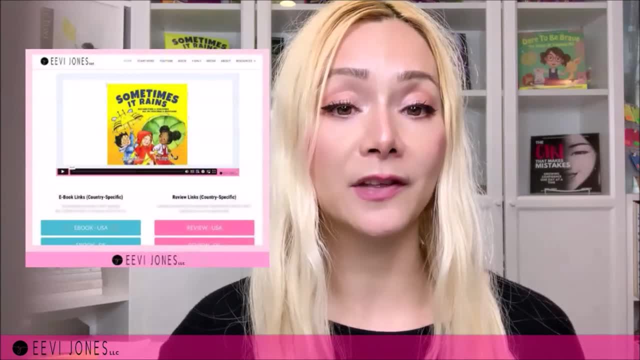 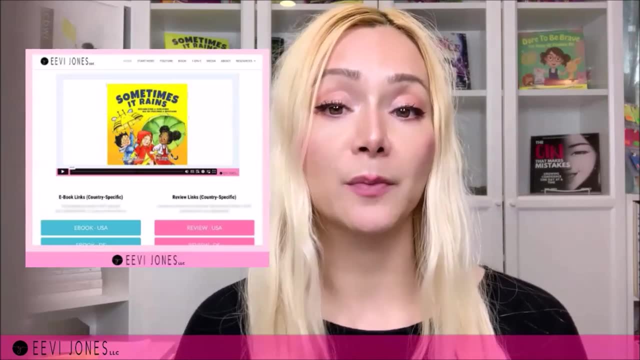 of my book and then share that with my launch team. For example, this right here is a website I shared with my launch team for my book Sometimes It Rains. It has a little note, shares my three minute Read Aloud video and links to the Amazon. 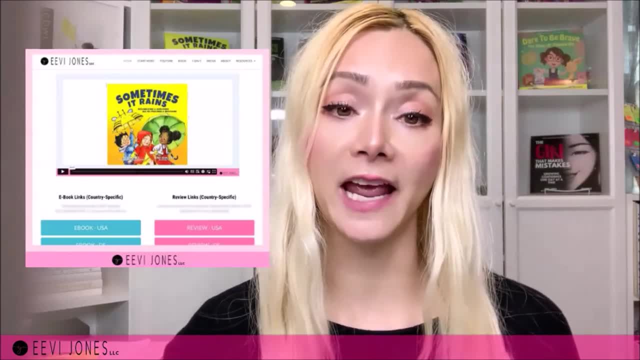 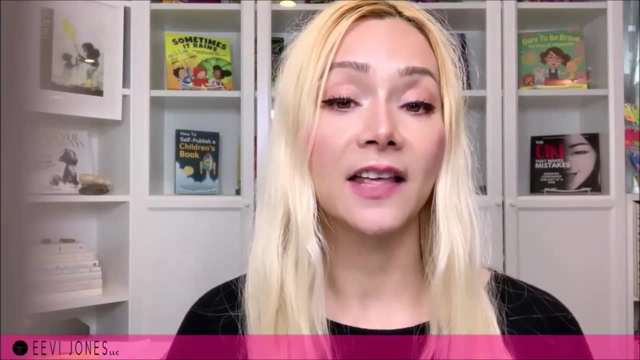 page, as well as a direct link to the review page over on Amazon. Now, if you would like to learn more about what a launch team is and how to use it- I have a separate video on just that that that I shared below- and if you would like to know how to create a, 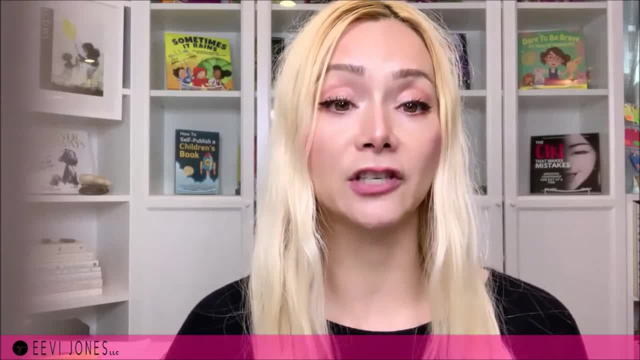 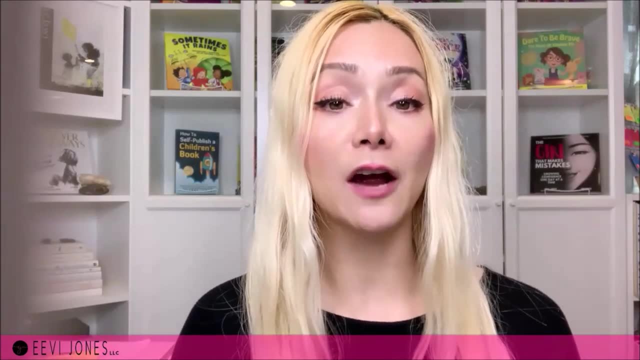 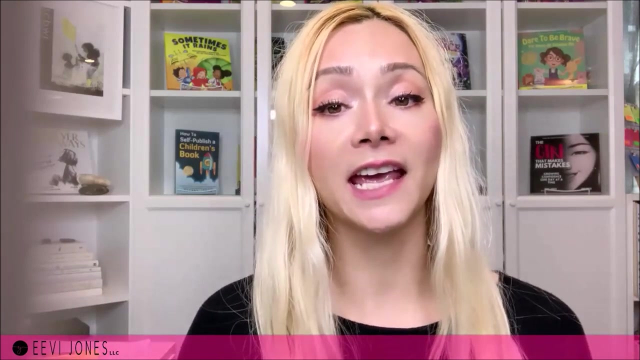 direct review link that takes people directly to the review page of our book. then I have a separate video for that as well, all shared in the description below, and so sharing our book that way makes it really easy and also fun for our launch team to read our book all in less than five minutes, so that they can then 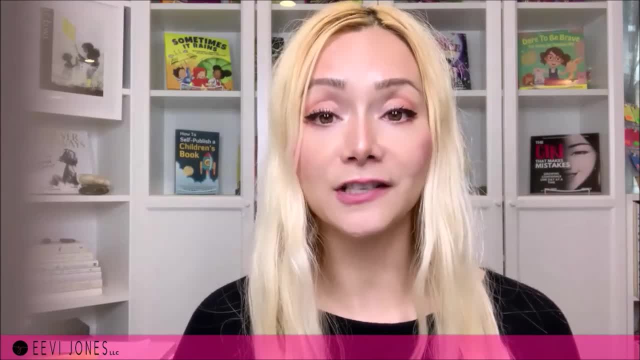 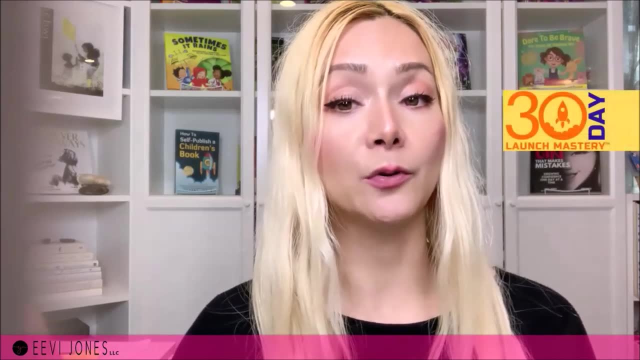 leave a review for us, and the easier we can make it for others the better, especially with everyone being so, so busy these days. if you're looking for a step-by-step launch strategy for your beautiful children's book, then make sure you check out my 30-day launch mastery below. it is one of my absolute favorite. 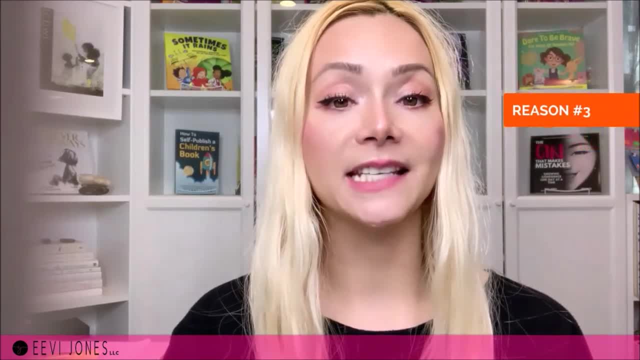 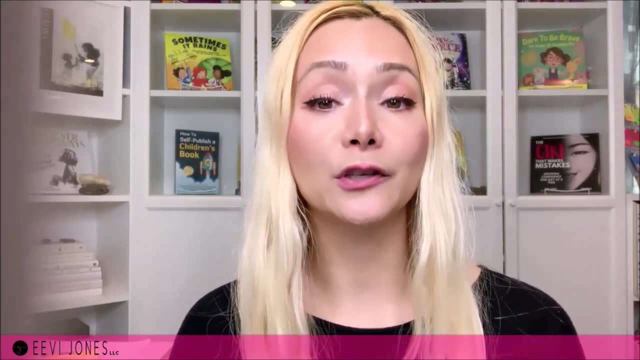 courses I have created over the years. and reason number three is that we can use a read aloud video of our book as an additional resource. when my boys were little, they loved it when I would read books to them and sometimes, when I was busy doing something else, I would give them one of their books and either play 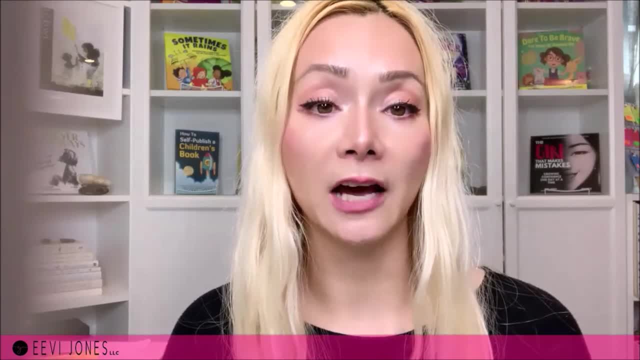 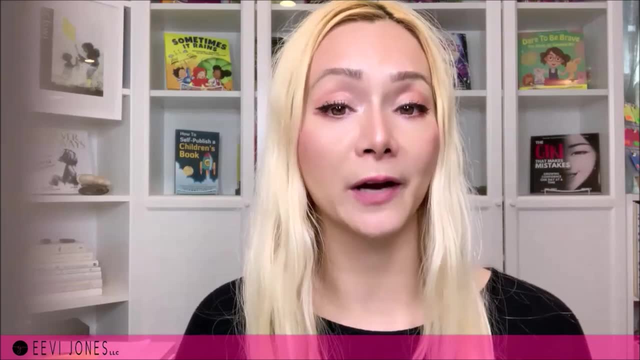 the audio book or play the audio book, or play the audio book or play the audio book version of it on repeat, or also a read aloud video. that way they would literally read along as they were turning the pages of their physical book while listening to the recording, and they loved doing that, and so what we as 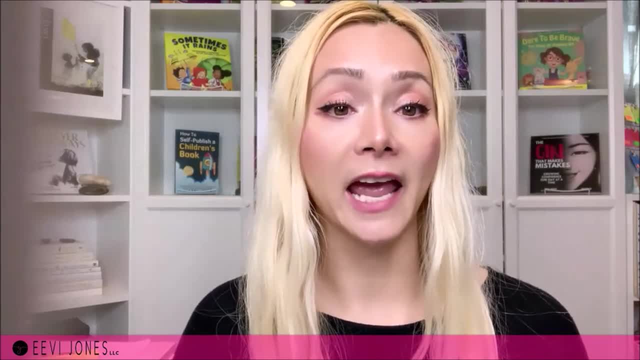 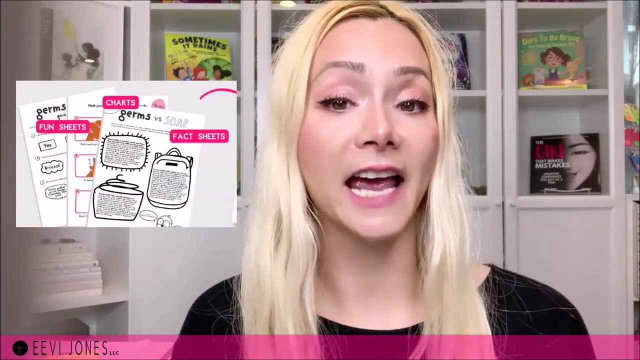 authors can do is offer a read aloud version of our book and, for example, only share it with those that have already purchased our book. if you have watched my video on final little extras we can create for our book, you already know why offering these final little extras can be really beneficial to your children's books. 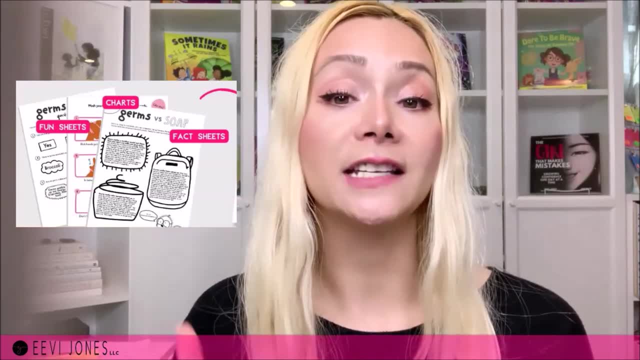 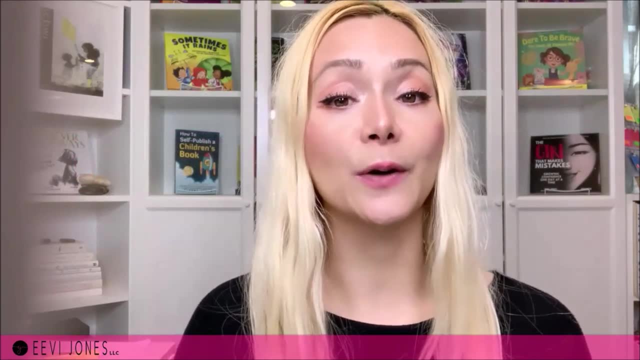 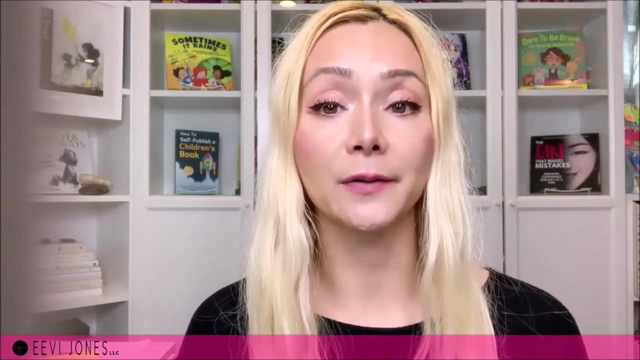 and so, besides extras like worksheets and coloring pages for our book, a read-aloud video can be another such resource. if you haven't seen that video yet, I will go ahead and add the link in the description below. so this is also a great alternative to the first option I mentioned earlier. so instead of sharing, 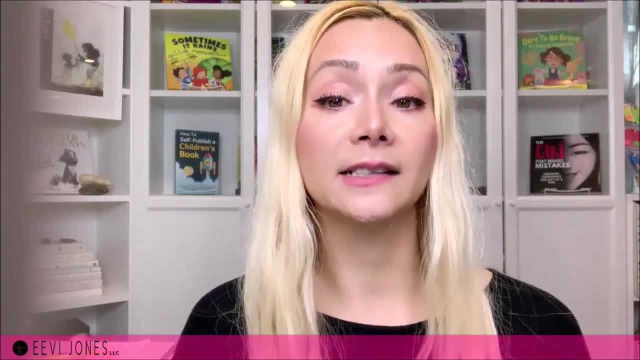 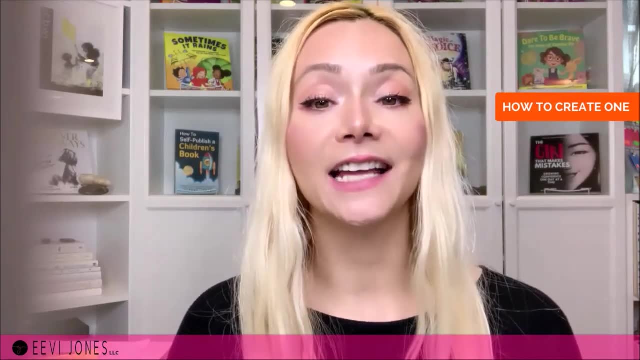 our read aloud video with everyone on YouTube. we can simply share it with just those who have already purchased our book. now that we have looked at the what and the why, look at the how, How can we create our very own read aloud video? As I already mentioned earlier, 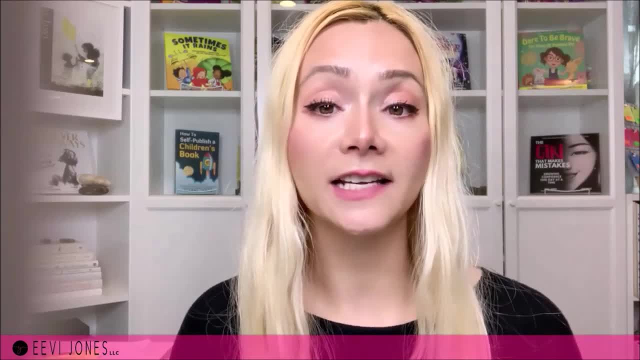 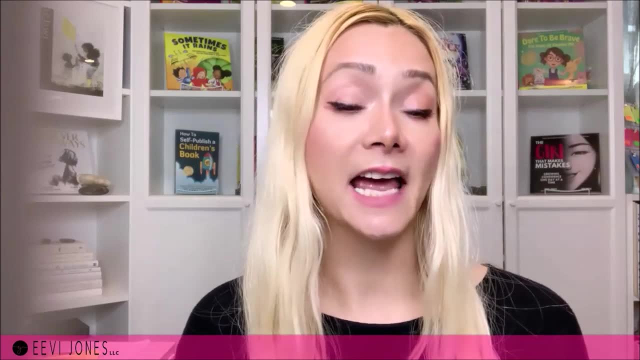 there are many different ways to go about this. The one I like a lot is where we see a realistic page turn effect. That way, moving from one page to the next feels less like a slideshow and more like the turning of the pages of an actual physical book, And so that's the method I'm going to share. 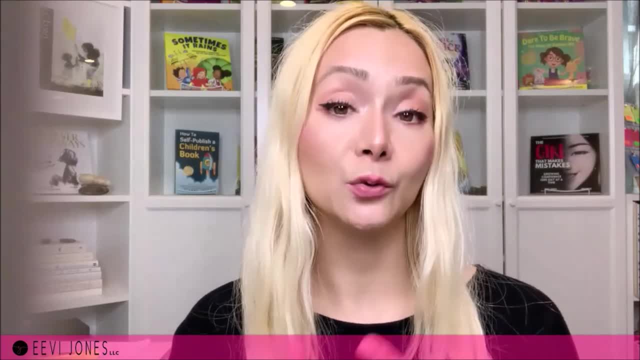 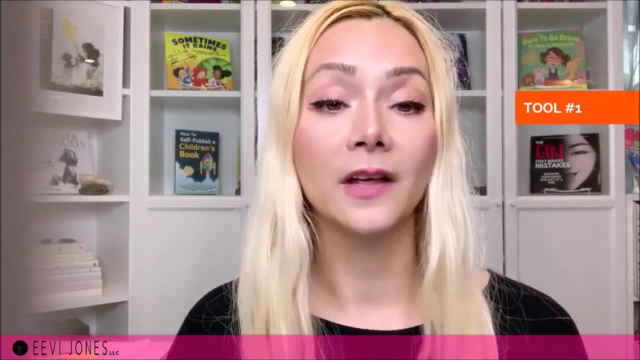 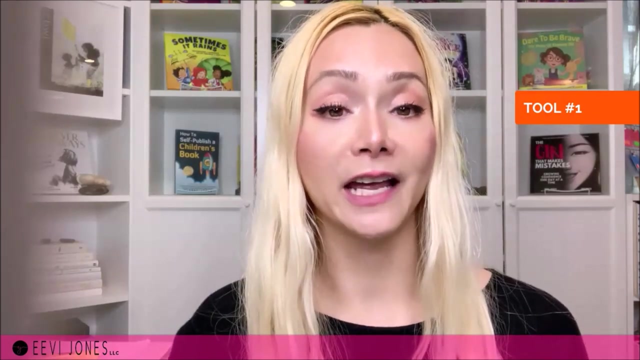 with you here To create a video like this. we will be using two tools, and the way we are using them, they will, as of right now, at the making of this video, be absolutely free. The first tool is called Hazine. That's a tool that will help us add the page turning effect that I was talking about. 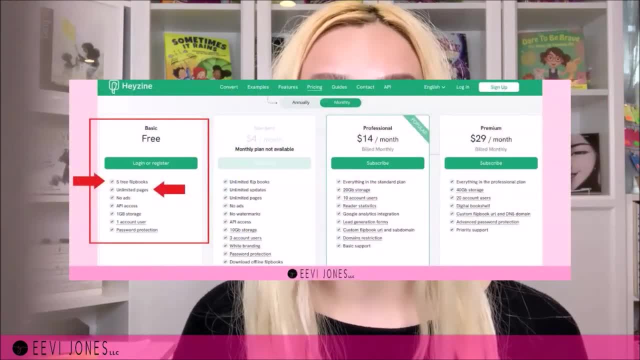 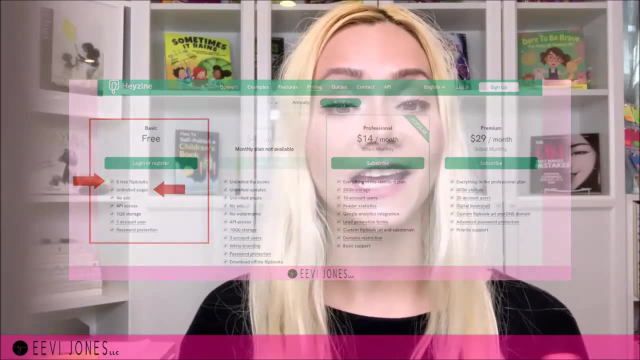 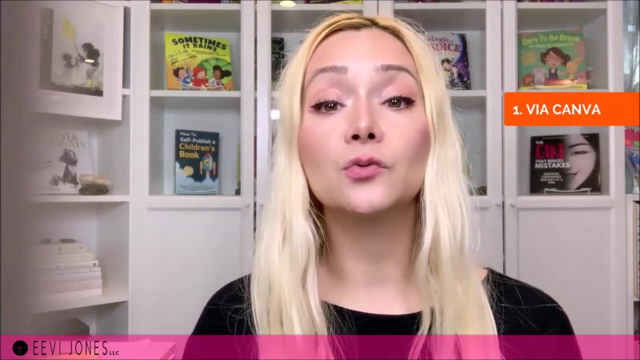 earlier. The basic plan is absolutely free and really all we need Right now. it allows us to make up to five flipbooks with an unlimited number of pages. All we need to do to use it is sign up Now. there are two ways we can use Hazine. The first way is directly through Canva, and this is 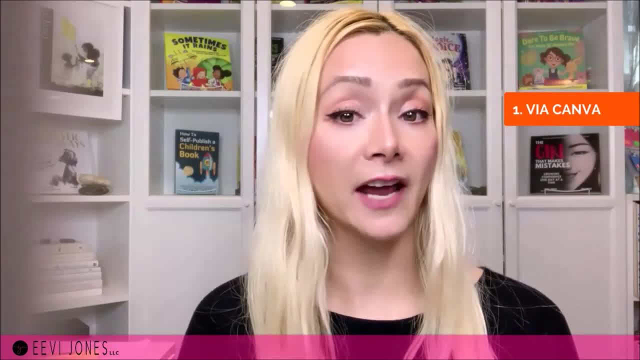 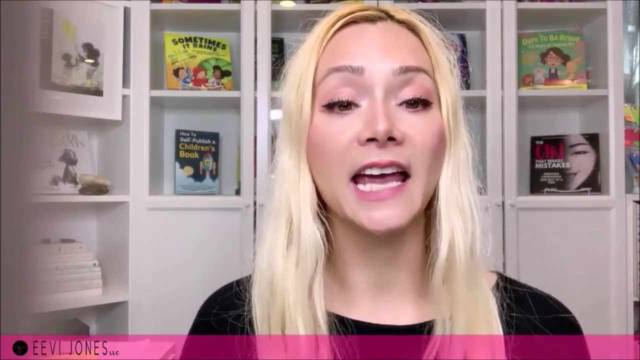 really helpful. If you want to learn more about how to use Hazine, you can go to the link in the description below. If you are already formatting our book in Canva anyway. So if, for example, you are already using my Plug&Go formatting templates to format your book, then using Hazine will be extra. 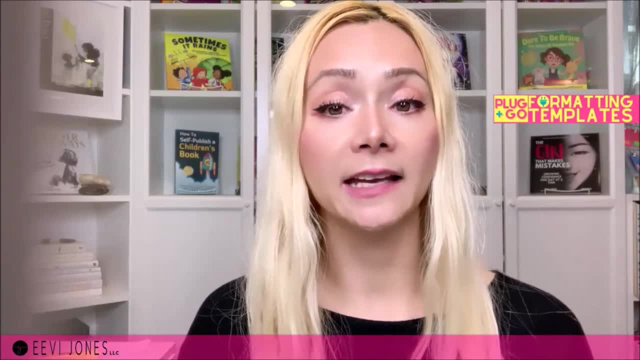 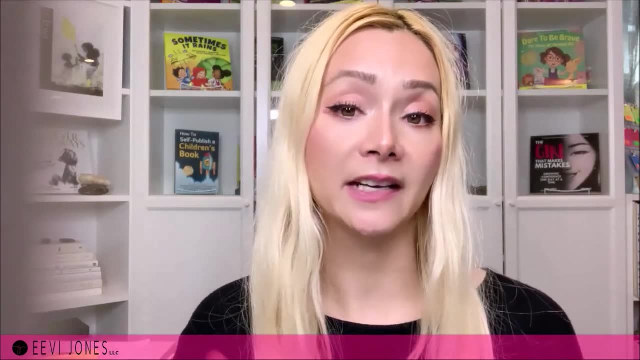 easy. I have shared the link to my Plug&Go templates in case you would like to use them to format the print version of your children's book. Sometimes it's a bit tricky to find the Hazine app in Canva, so I went ahead and shared the direct link to Hazine in Canva in the description below. 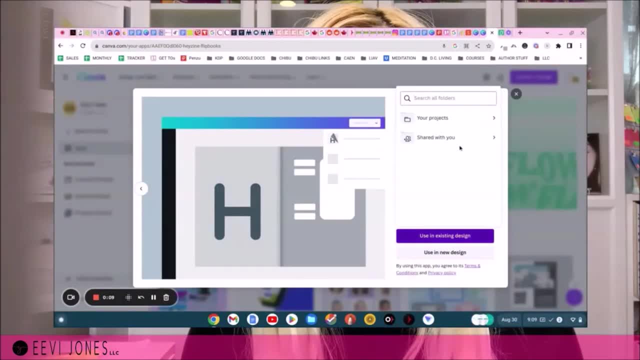 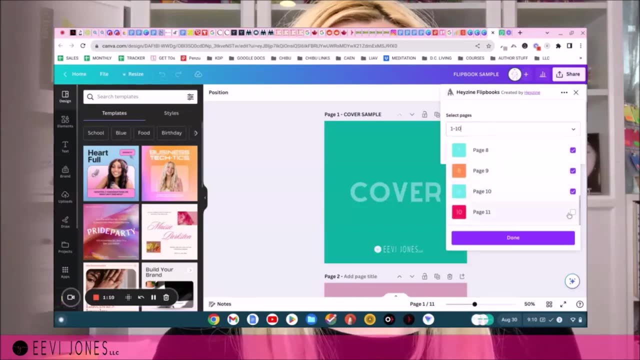 When we click on that link, it will open the Hazine app and we will be able to see the design directly in Canva, where we can then click on the use an existing design, which then lets us choose our design or project from a drop-down menu. This will open our project with another. 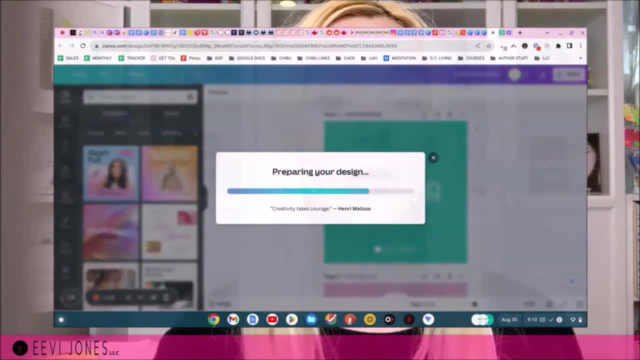 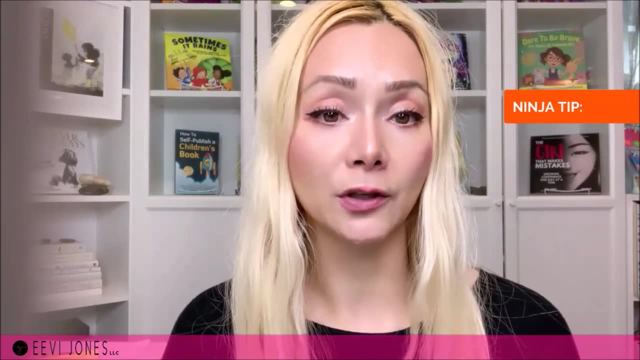 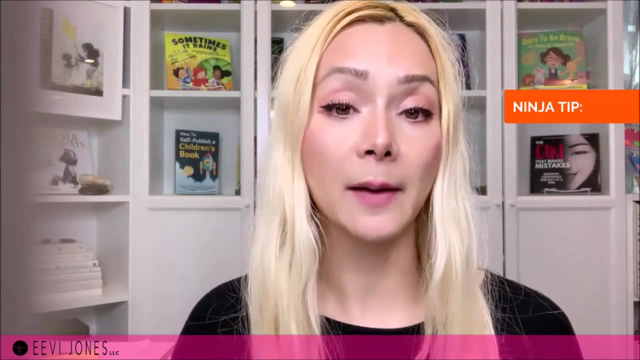 drop-down menu where we can choose what pages we would like to include in our flipbook. Now here's my first ninja tip when using Hazine. Usually, the interior file of our children's book does not include our cover page, but if we want our flipbook to show our cover page, we need to temporarily add. 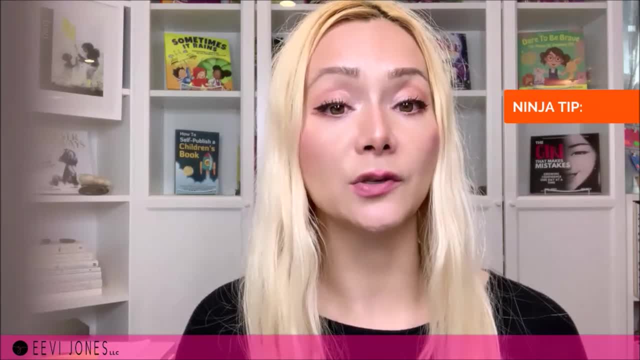 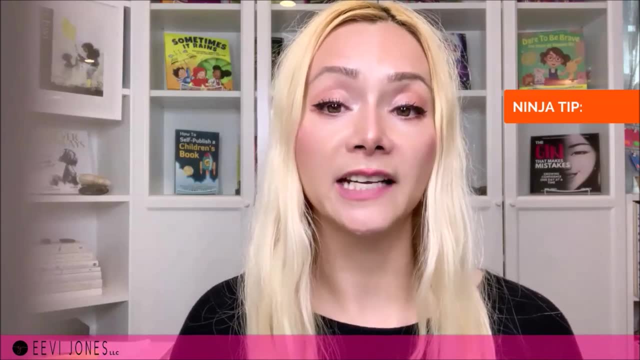 a cover page to our book. If we want to show our cover page, we need to temporarily add a cover page to our Canva project here. So that is what you see here as well. The first page is a cover page. but again, that cover page is here only temporarily and we will want to delete it once we are done with our 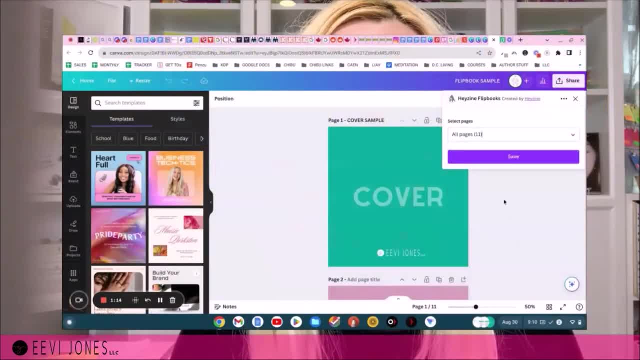 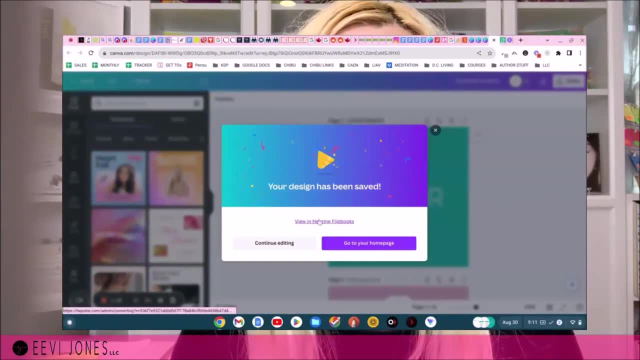 flipbook. So once we have all pages selected, we can click save. and once we see the confirmation box that our project has been saved, we simply click on view in Hazine flipbooks right here, which then will open our created flipbook where we can now flip through our pages. The second way of 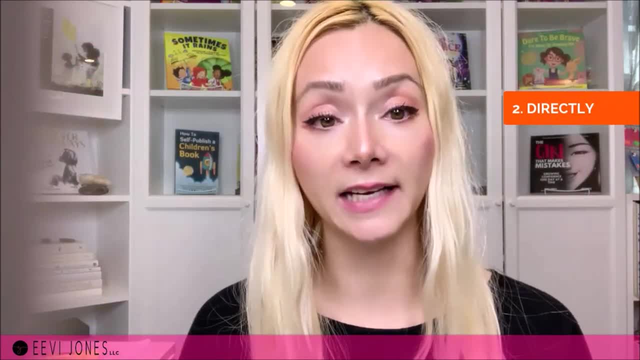 using Hazine is just to click on the save button and then click on the save button and then click on the save button. The second way of using Hazine is just to go to Hazine's website directly. So if, for example, you already have your formatted pdf file of your beautiful book, then we can upload that pdf over. 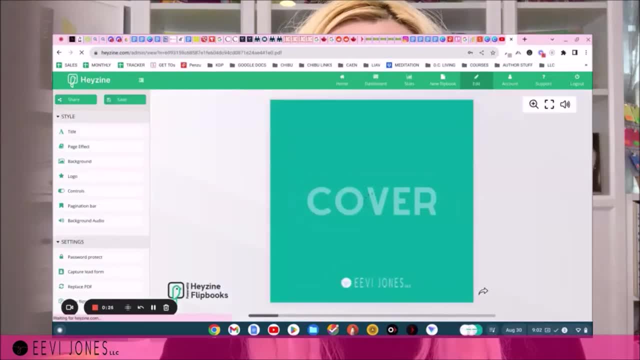 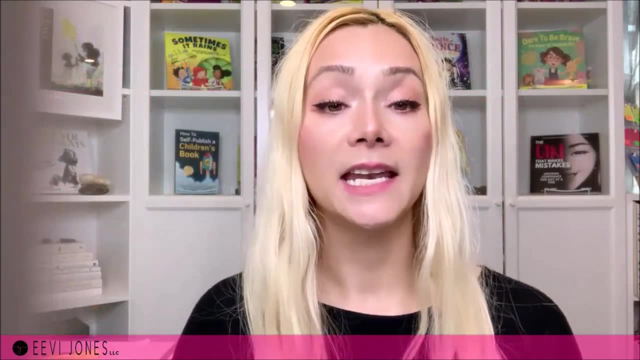 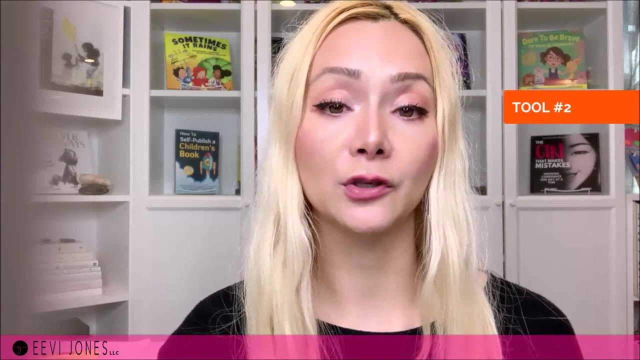 on Hazine directly and it will convert into a flipbook. But remember, if we want our flipbook to show our cover, it must be part of the pdf we are uploading. Now that we have the page turning effect, it's time for our second tool, and that is loom. Loom will allow us to record our screen. 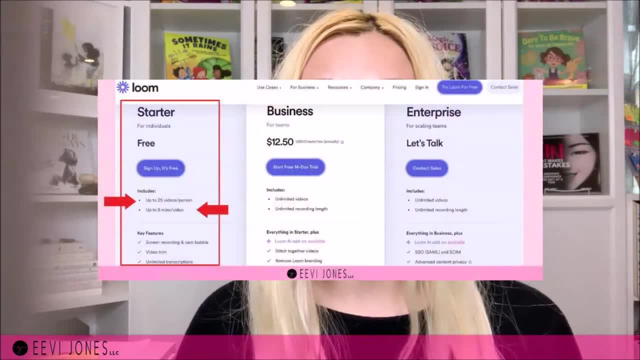 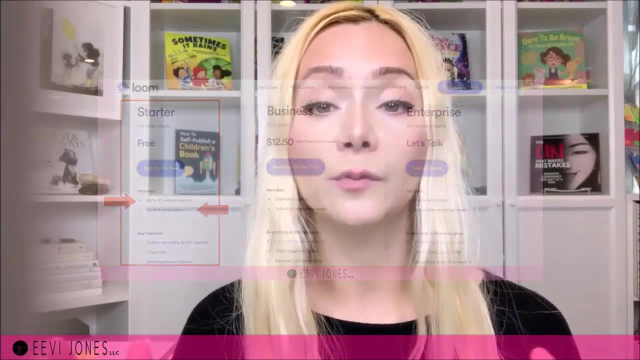 as we are reading our book aloud. The basic way to record our screen is to click on our flipbook. The basic plan, again, is absolutely free Right now. it allows us to make up to 25 videos that can be up to five minutes long, and that will be more than enough for our needs. All we need to do to use it. 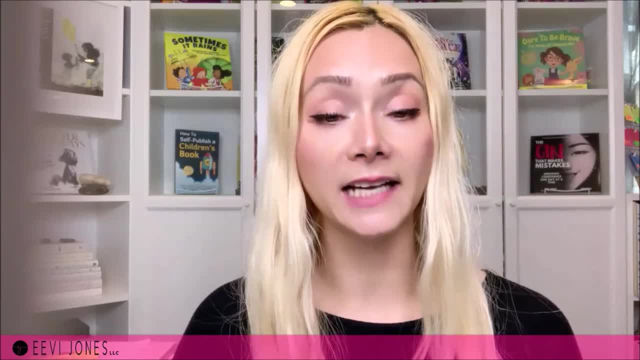 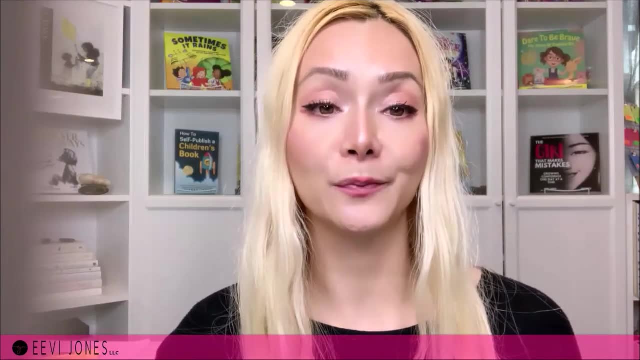 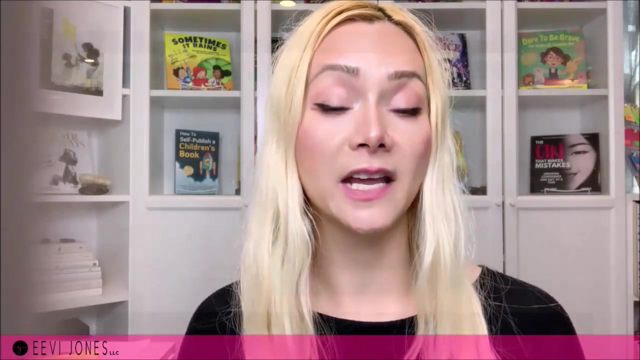 is to sign up for it. We will be recording our flipbook directly in Hazine. so once you have signed up for a loom account, it will walk you through how to start recording your first loom Here. I was recording my laptop so you can see how I was screen recording my read aloud. So with our flipbook open, 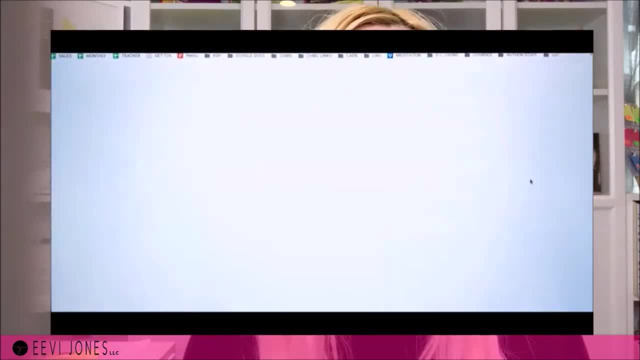 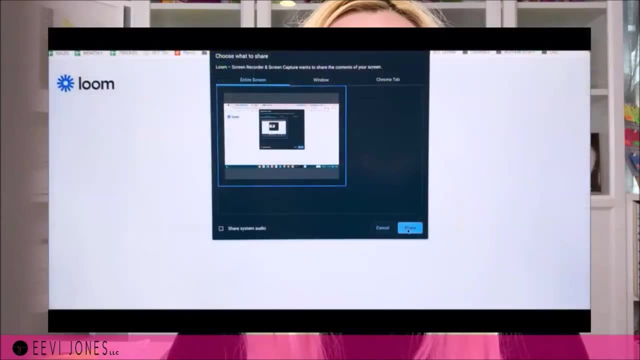 we simply begin screen recording. First we get to choose the screen size we want to record. I usually choose full screen here, so it captures the entire screen. I click on start recording and confirm what area I want to record one more time and then we'll see a little countdown In Hazine. 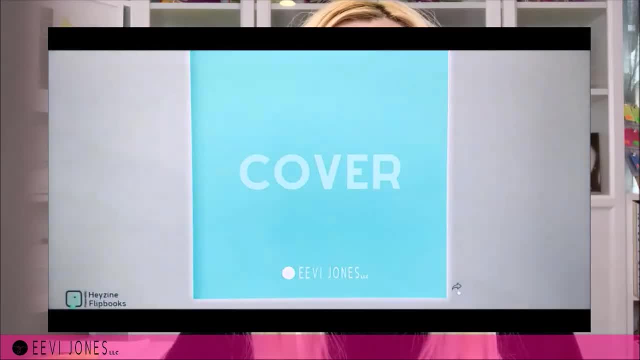 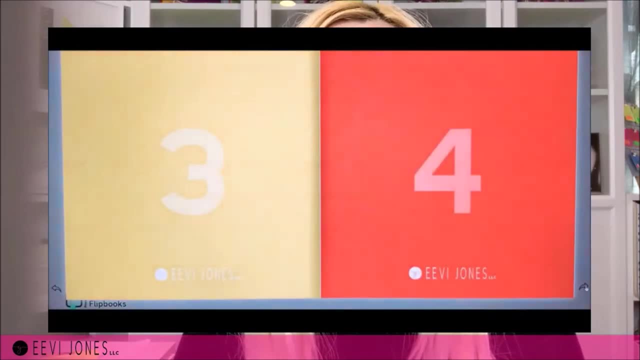 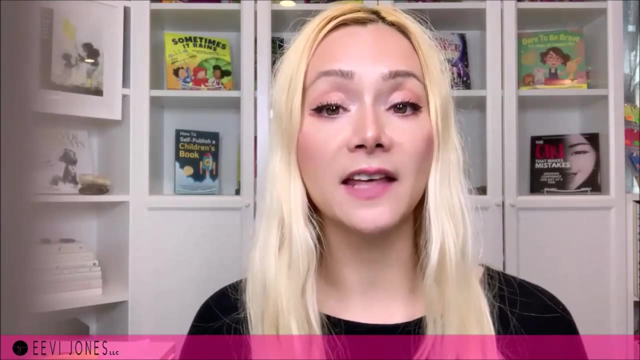 we will want to click on the full screen option as well, so our flipbook expands across the entire screen and that's where we can begin reading our book aloud, where it records our voice as well as flipping through them. Now, if you make a mistake, don't worry, we can edit that out right after we. 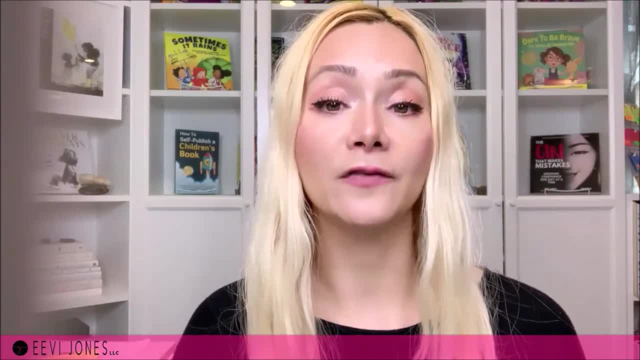 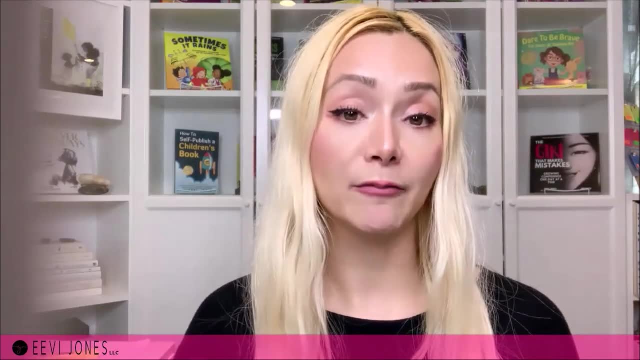 are done recording. That's the beauty of loom: it lets us edit our video right then and there. Remember that our video must be less than five minutes long, so make sure you're pacing yourself properly. I usually don't take more than three to four minutes. 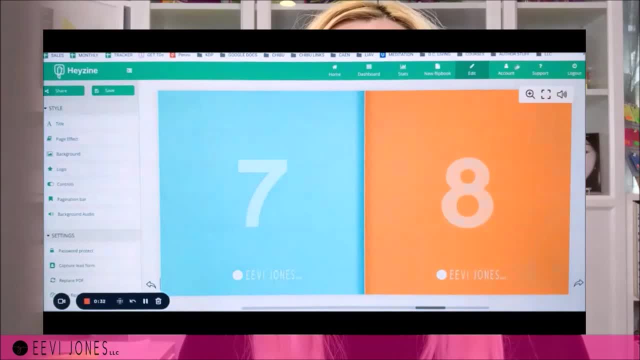 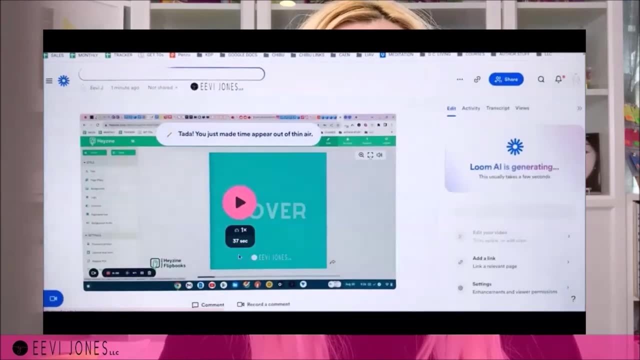 reading my books. Once we are done reading our book, we can simply exit the full screen mode and stop our screen recording by clicking the stop button in the bottom left corner. Our recording is automatically opened over on loom, where we can now edit our video by clicking on.